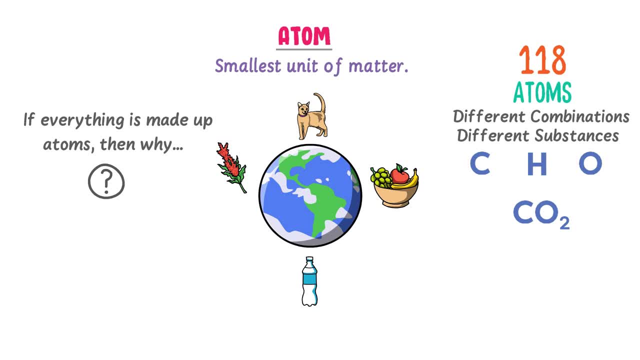 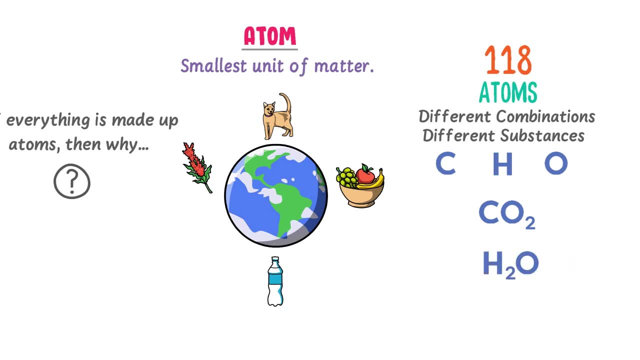 Carbon and oxygen combine together chemically, they form carbon dioxide gas, CO2.. When hydrogen and oxygen combine together chemically, they form water, H2O. Thus, different combination of atoms produces different substances. Now coming to the difference between atom, element, molecule and compound. 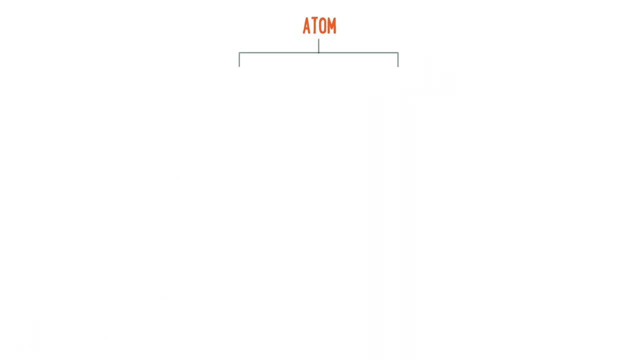 There are two main type of atomic combinations: homo-atomic combination and hetero-atomic combination. The word homo means same and atomic means atom. So the word homo-atomic means same type of atoms. Now, when an atom or group of atoms exist freely, it forms a molecule. 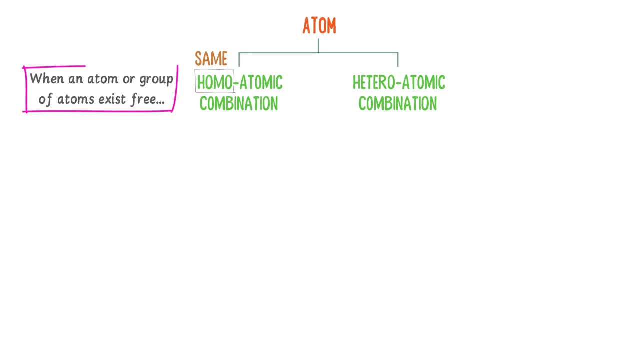 Let me repeat this important statement: When an atom or group of atoms exist freely, it forms a molecule. For instance, homo-atomic combination of atoms form a molecule. In homo-atomic combination of atoms, molecule will be either mono-atomic molecules or diatomic molecules. 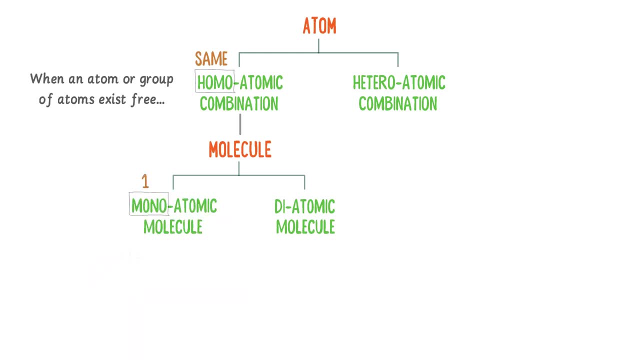 The word mono means one, So mono-atomic molecules are like neon, argon and xenon. One can say that all noble gases form mono-atomic molecules Because they are made up of only one atom. Now, when many mono-atomic molecules combine together, they form element. 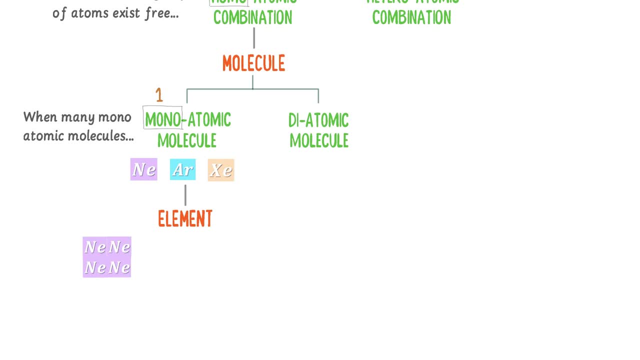 For example, when many atoms of neon combine together, they form neon element. When many atoms of argon combine together, they form argon element. When many atoms of xenon combine together, they form xenon element. Similarly, when many atoms of metal 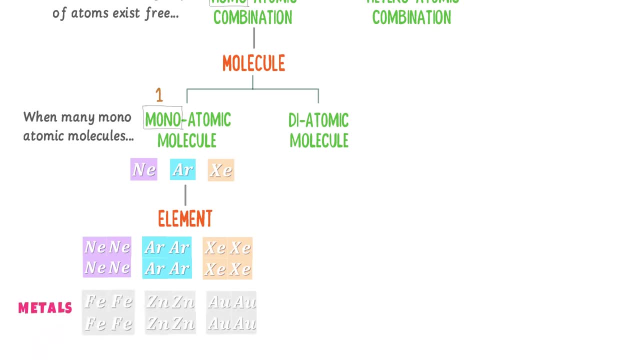 Like iron, zinc, gold etc. combine together, they also form elements. But remember that metals like iron, zinc and gold do not form molecules. Now the word di means two, So diatomic molecules are H2, O2 and N2.. 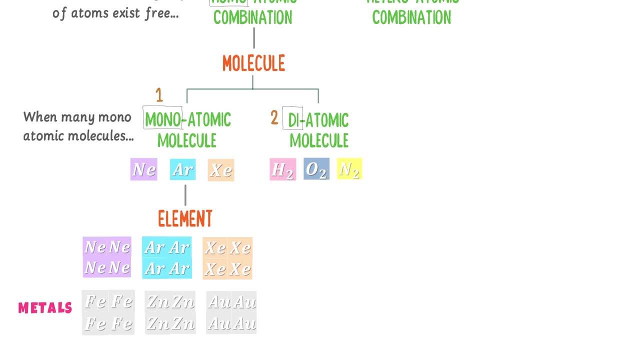 They are made up of two atoms. That's why we call them diatomic molecules. These types of molecules are also called as elemental molecules. When many elemental molecules combine together, they also form elements. For example, when many elemental molecules of H2 combine together, they form hydrogen element. 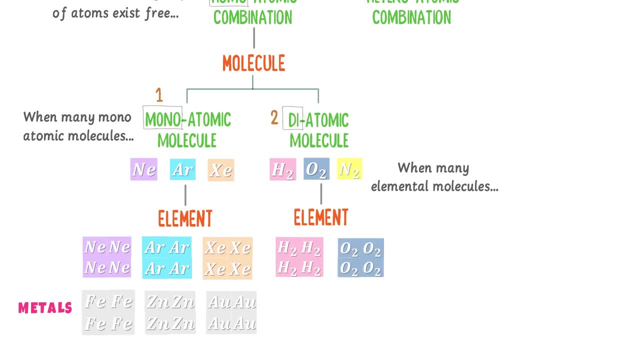 When many elemental molecules of O2 combine together, they form oxygen element. When many elemental molecules of N2 combine together, they form nitrogen element element. Therefore, remember that Neon, Argon and Xenon are monoatomic molecules because they exist freely in the nature, while H2, O2 and N2 are diatomic molecules because they 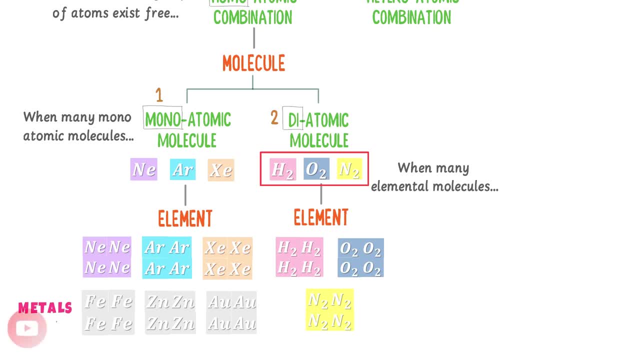 can also exist freely in the nature, But one atom of Hydrogen, Oxygen and Nitrogen do not exist freely in the nature. On the other side, elements are formed due to homoatomic combination of either atoms like neon, iron or gold, or it is formed by elemental molecules like H2,. 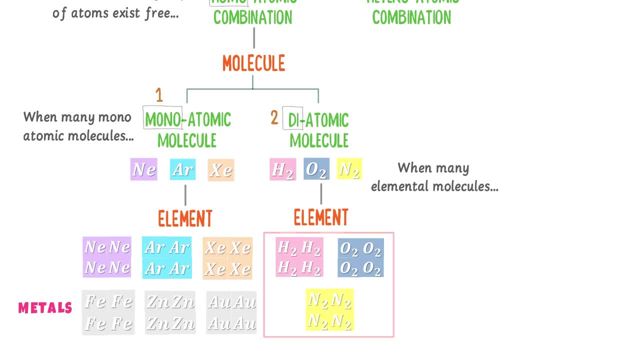 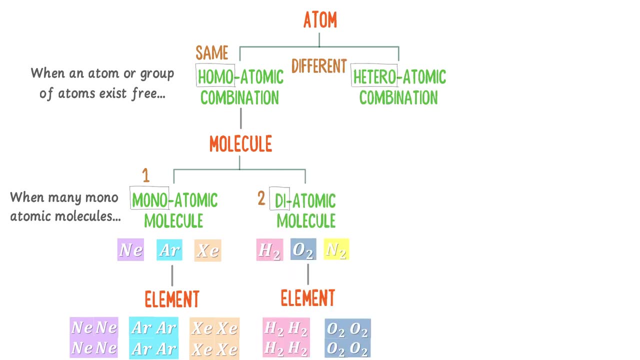 O2 and N2.. Now coming to the heteroatomic combination of atoms. The word hetero means different. heteroatomic combination means when different atoms combine together chemically the other atom becomes homogeneous. gets the value When different atoms combine together. 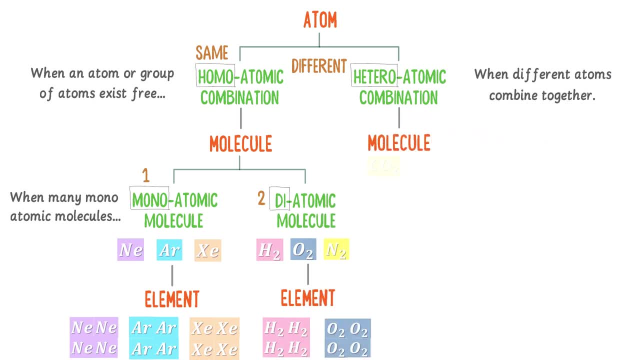 the atom is completely different from other atoms. To find the value, we need to consider also form heteroatomic molecules, For example, like CO2, H2O and CH4.. CO2 are formed from carbon and oxygen, H2O are formed from hydrogen and oxygen And CH4 are formed from carbon. 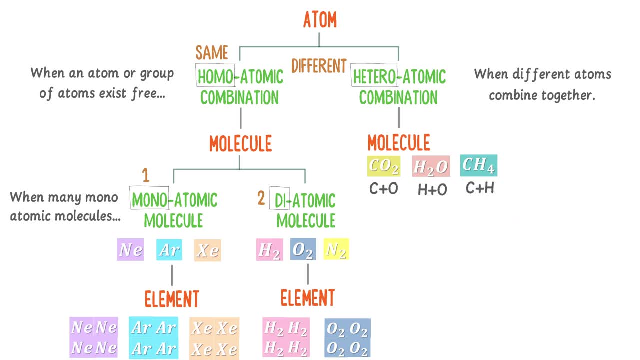 and hydrogen. That's why we call them heteroatomic molecules. Now, when many heteroatomic molecules combine together, they form a compound. For example, when many heteroatomic molecules of carbon dioxide gas combine together, they form compound of carbon dioxide gas. When,